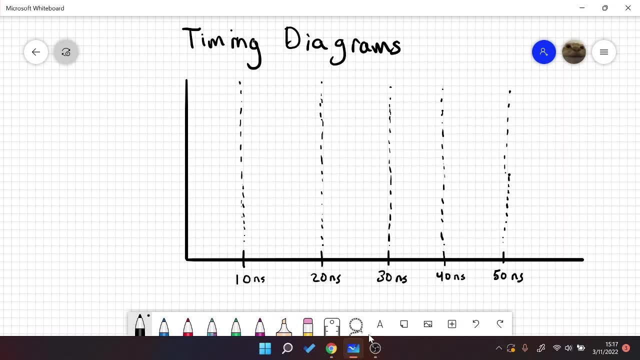 Hello. so today we're going to be doing a quick overview of timing diagrams. I'm going to talk about a little bit of timing diagram, how to do one, how to handle delay, and we're just going to do a very simple circuit, because I will cover timing diagrams for flip-flops in a different. 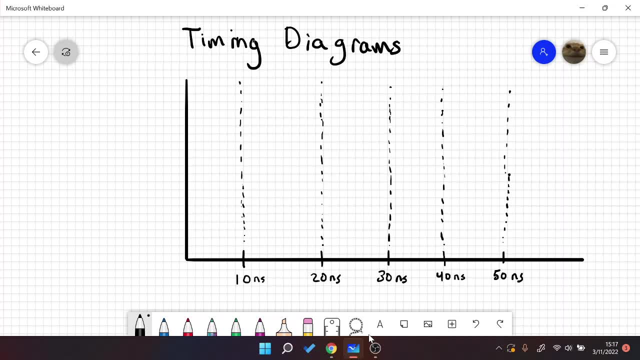 video. So for this video I have a timing diagram pre-made here. Excuse the little slop on the right side, but we're going to basically, let's come up with a combinational logic circuit and we're going to put that on a timing diagram. So let's take the circuit: a, b plus c equals y. 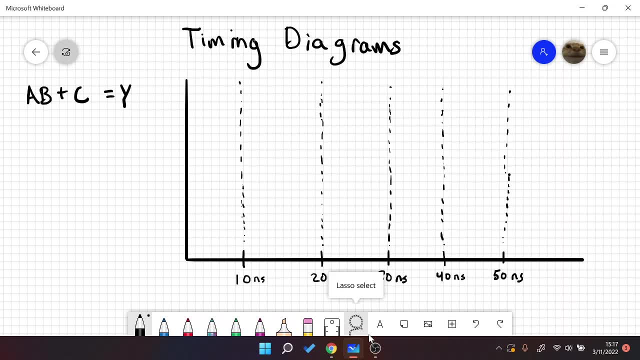 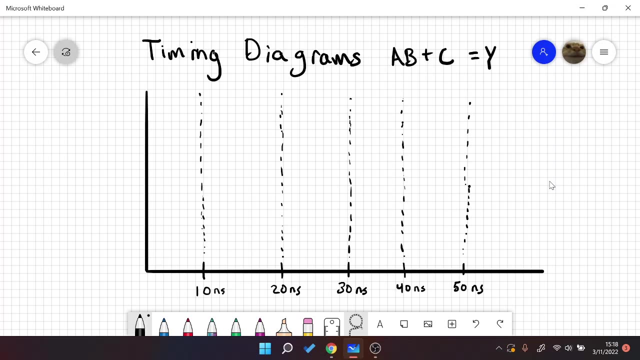 So actually, let me move that up here, Let's move that up there. So we have a, b, c plus y. That's what we're working with, Or a, b, c. a b plus c equals y, sorry. So first let's define our signals. a. 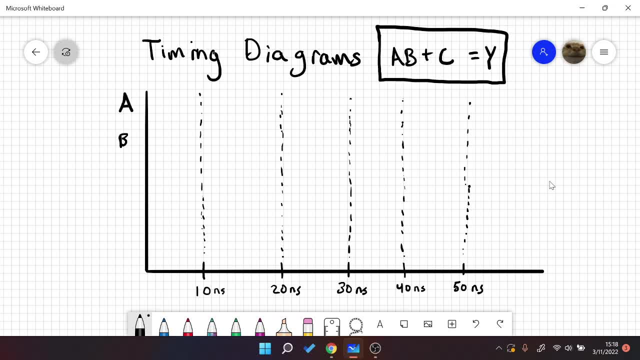 b and c. These will most likely be given to you randomly, or they'll ask you to find the signals a, b and c. from y, They'll give you the signal y. So let's say, these signals are something like this: 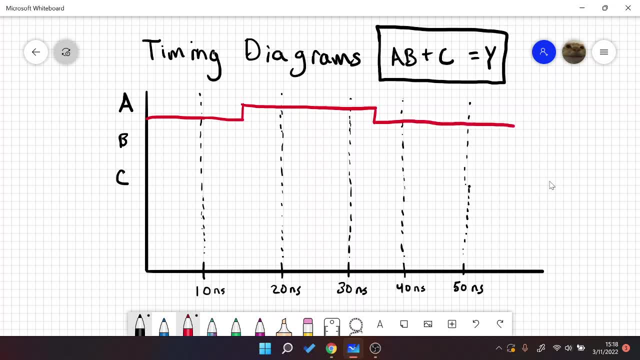 We'll do something like this. And finally, for c, we'll do something like this: Okay, so the first step to figuring this out is we need to find a- b. So let's find a- b. So we know that this signal is a and b. So what that means is, according to our truth, table for 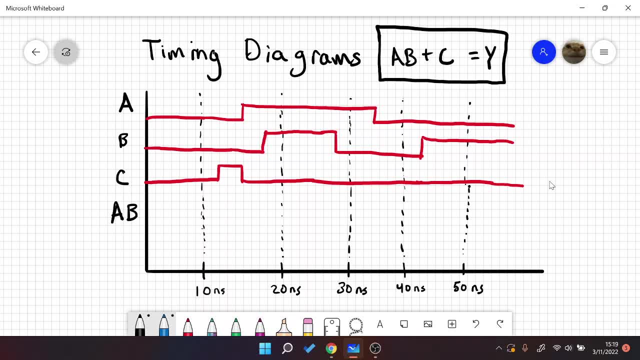 a and b. we know that this signal should only be high when a and b are equal to a, So we need to find a and b or both one. So a and b are both one, starting at this point, right here. So let's. 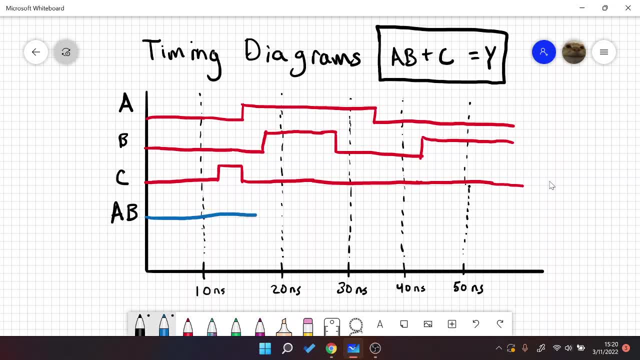 show that. So it should start low And when there's this signal we should go high. But let's say, if our problem has a little bit of delay, let's say that we need to account for five nanoseconds of delay for each gate. then we need to show about five nanoseconds of delay. 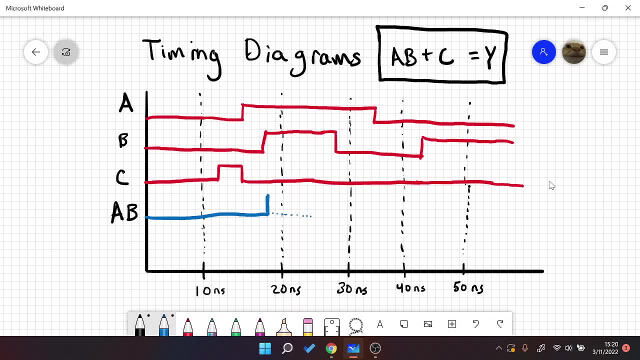 So what that would look like is: you would have something like this and something like that, So that would account for your delay. Your delay would also happen when it goes down. But let's just for now keep in keeping with no delay. So we're going to draw a line here. 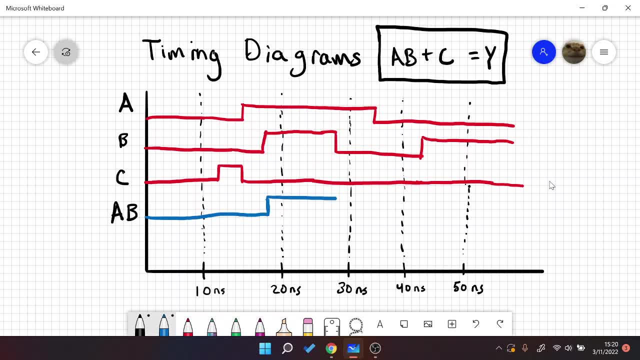 all the way to here. And this is when b drops, So our delay should go down here. And when b rises, a is not high, so it just stays low. So that's our signal. for ab, Now we know we can find ab plus c for y, So let's do this in green. 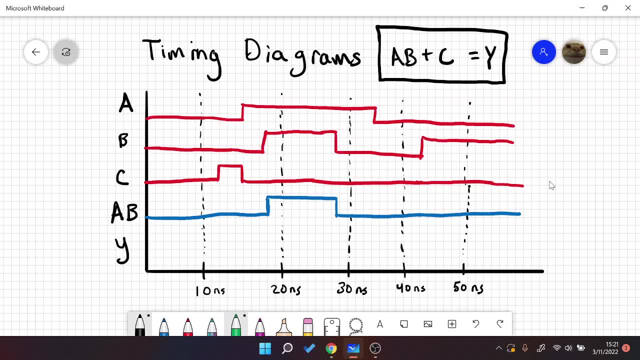 So we know that ab plus c should be one Whenever either of these two signals, c or ab, are one. So our signals start low, so we should start low, And then, when c goes high, we make this go high, And then it drops here And then it picks up again here. 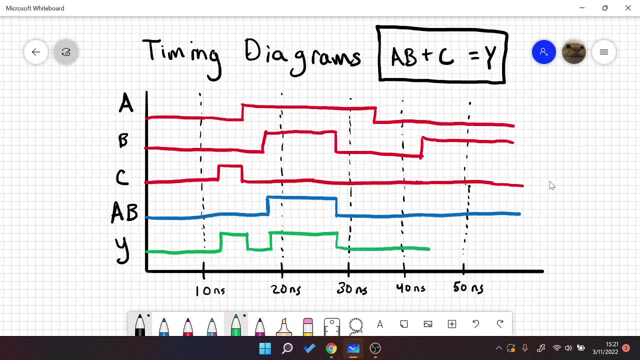 And then drops here again And then we're low for the rest of the circuit. So that is your basics of timing diagrams for a combinational logic circuit. I will go over something more advanced in our flip-flop timing diagrams video.